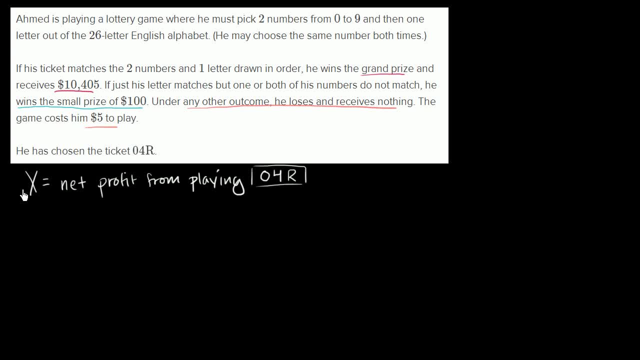 So Amit's particular ticket right over here. So let's just say x is the random variable, It's the net profit from playing this ticket. What I want to think about in this video is: what is the expected value of that? What is the expected value of that ticket? 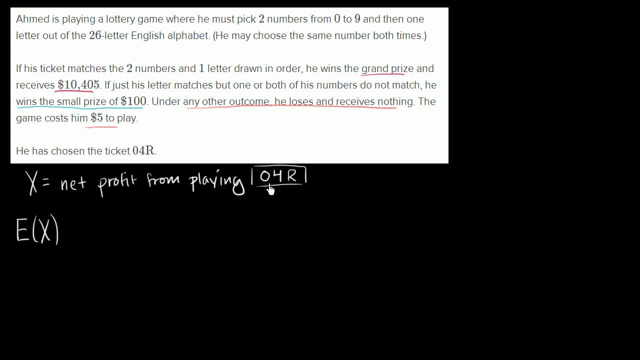 What is the expected net profit from playing 04R? And I encourage you to pause the video and think through it on your own. So let's think about what expected value is. It's the probability of each of those outcomes times the net profit from those outcomes. 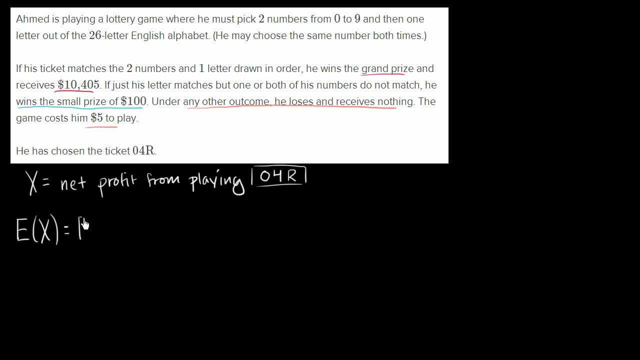 So there's the probability of the grand prize. Let me do that in that red color. So there is the probability of getting the grand prize. And now, what would times his net pay? What's the net payoff from the grand prize? What would that be? 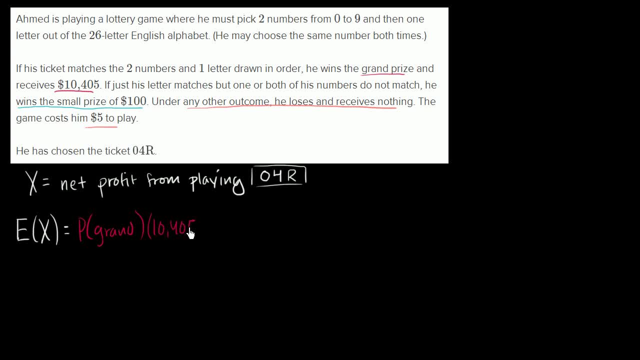 Well, he gets $10,405, but that's not his net payoff or his net profit. I should say His net profit is what he gets minus what he paid to play. So he paid $5 to play. So this would be so, that's that. 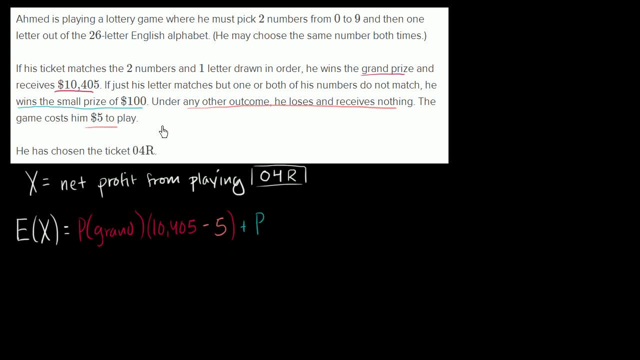 So plus plus the probability of getting the small prize, probability of the small prize plus the payoff of the small prize, which is going to be $100, or times the net profit. I guess, if you get the small prize, So you get a payoff of $100 minus you have to pay $5 to play. 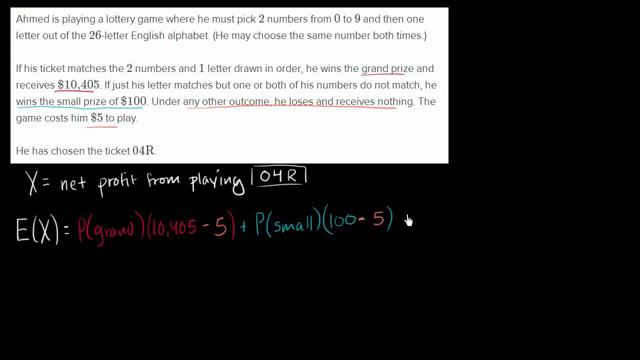 And then, finally, you have the probability of neither. So you're essentially not winning. And there, in that situation, what is the net profit? Well, in that situation, your net profit is negative 5. You paid $5 and you got nothing in return. 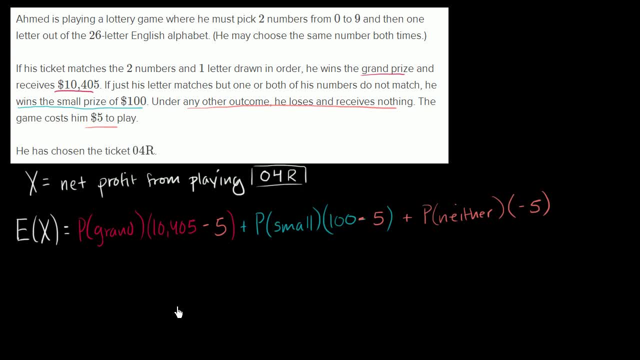 So to figure out the expected value, you just have to figure out these probabilities. So what's the probability of the grand prize? Let me do that over here. Probability of grand prize: Well, the probability that he gets the first letter right is 1 in 10.. 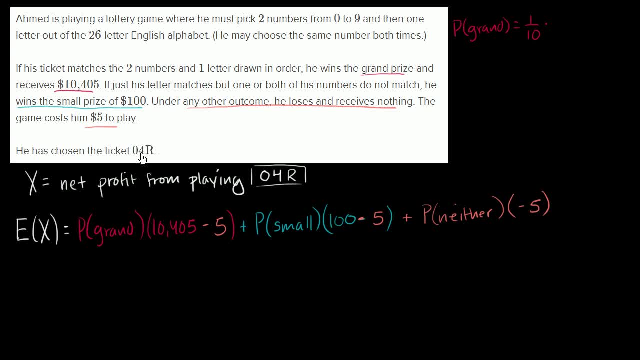 There's 10 digits there. Probability that he gets the second letter right is 1 in 10.. These are all independent And probability that he gets the letter right. there's 26 equally likely letters that might be in the actual one. 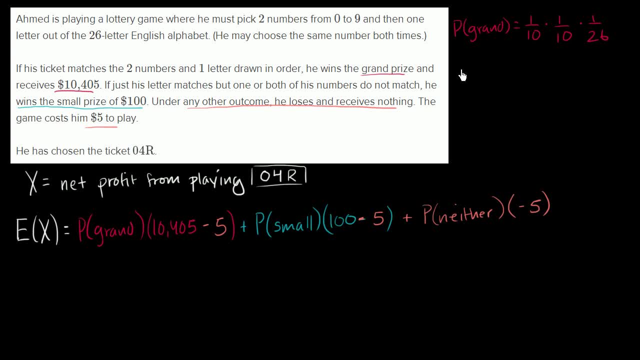 so he has a 1 in 26 chance of that one. So the probability of the grand prize is 1 in what is this? 2600.. 1 in 2600.. So this is 1 in 2600.. 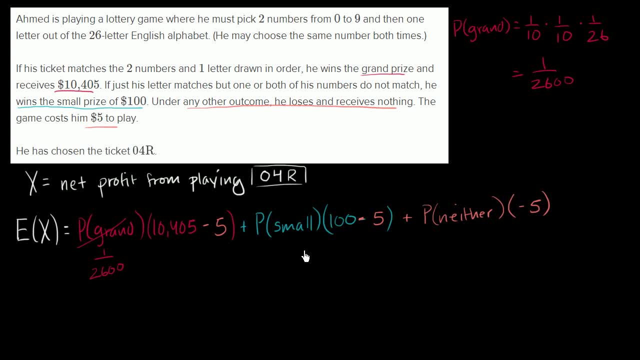 Now, what's the probability of getting the small prize? Probability of the small prize? Well, let's see He has a 1 in 26 chance. The small prize is getting the letter right. Getting the letter right, But not getting both of the numbers right. 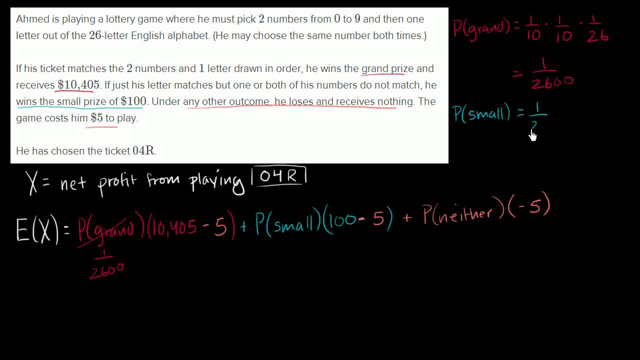 So he has a 1 in 26 chance of getting the letter right. But this isn't. we're not done here, just with the 1 in 26. Because he has a 1 in 26,. this 1 in 26,. 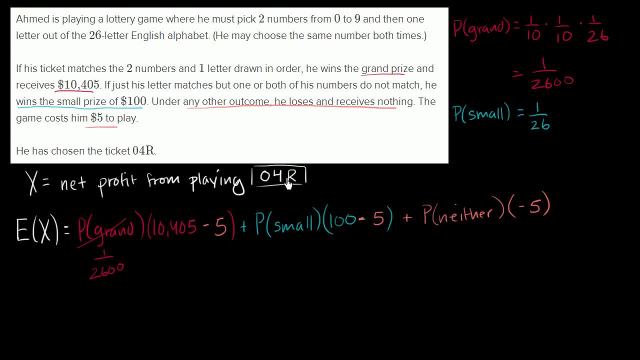 this includes all the scenarios where he gets the letter right, including the scenarios where he wins the grand prize, where he gets the letter and he gets the two numbers right. So what we need to do is we need to subtract out the situation, the probability of getting the two numbers. 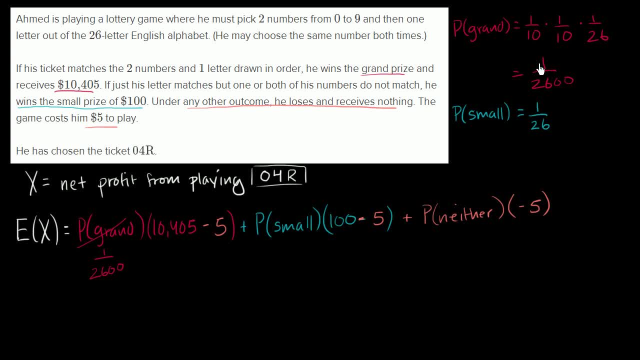 getting the letter and the two numbers right, And we already know what that is: It's 1 in 2600.. So it's 1 in 26 minus 1 in 2600.. The reason why I have to subtract out this 2600 is: 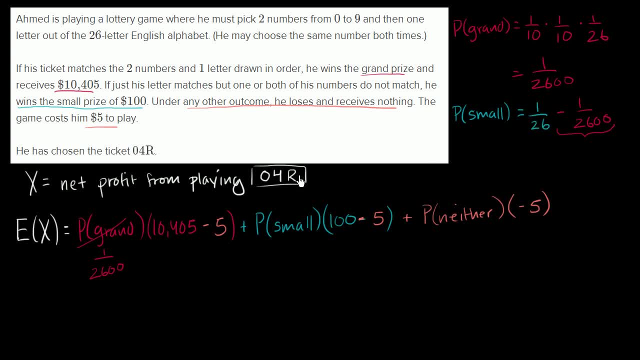 he has a 1 in 26 chance of getting this letter right. So that includes the scenario where he gets everything, Where he gets everything right. But the small prize is only where you get the letter and one or none of these. If you get both of these, then you're in the grand prize case. 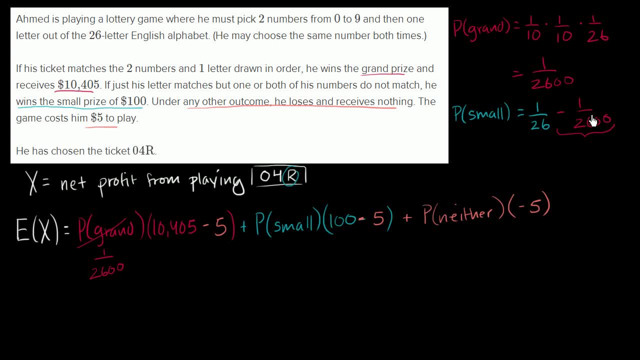 So you essentially have to subtract out the probability that you won the grand prize, that you got all three of them to figure out the probability of the small prize. Now, what's the probability of essentially losing The probability of neither, The probability of neither. 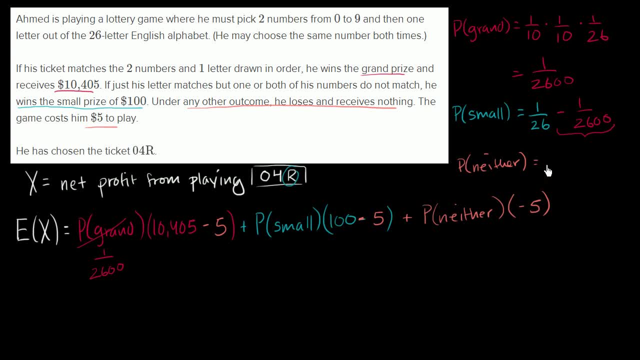 Well, it's just kind of, you know, that's everything else. So it would be 1 minus these probabilities right over here. So it would be 1 minus these. The probability of the small prize. The probability of the small. 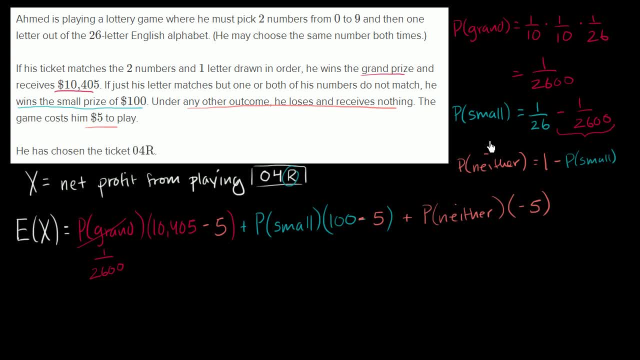 Minus the probability of the grand. These are the possible outcomes, So they have to add up to 1 or 100%. So this is 1 minus probability of small, minus probability of large, Minus probability of large, Or I said not grand prize. 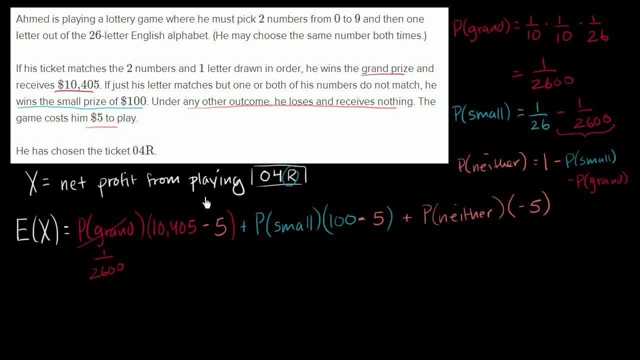 Grand prize. So let's fill this in. So the probability of the small one- I'm using that red too much- This right over here is 1 in 26 minus 1 in 2600.. 1 in 2600.. 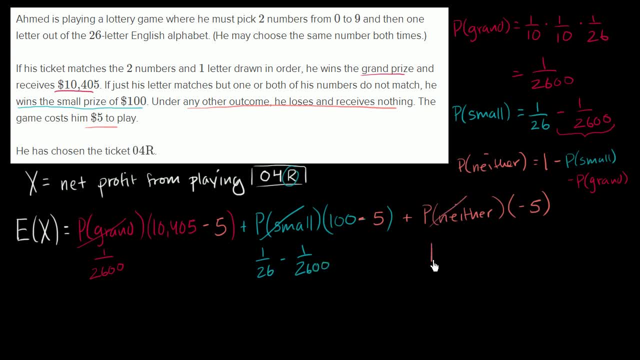 And then this right over here is 1 minus the small, which is 1 in 26 minus 1 in 2600.. Minus 1 in 2600.. Minus 1 in 2600.. And this simplifies to. 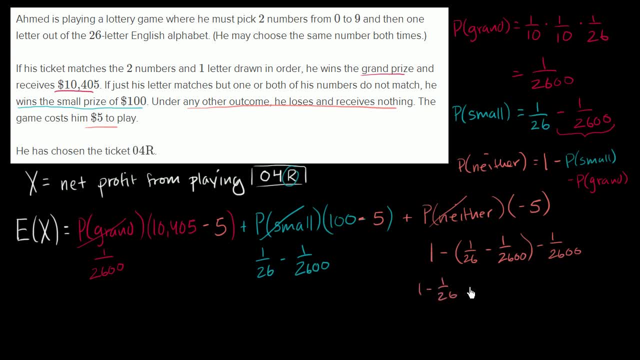 Let's see This is 1 minus 1 over 26. Plus 1 in 2600.. Plus or minus 1 in 2600.. These cancel And you're left with 1 in 1 in 26.. Now, why does this make sense? 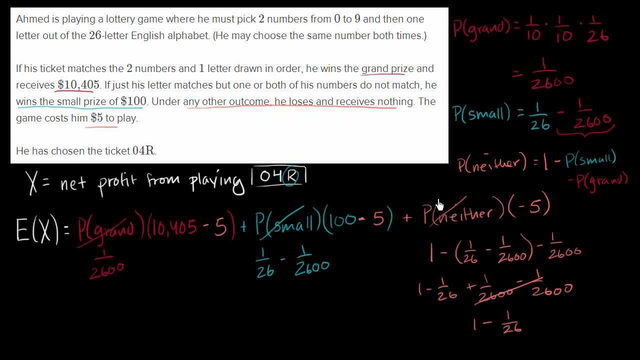 Well, the way you lose, The way you get nothing, is if you get the letter wrong. So if you get, You have a 1 in 26 chance of getting the letter right, And then you're going to be in one of these two categories. 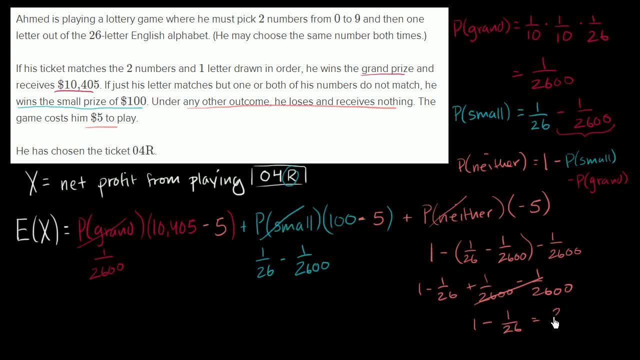 Or you have a 1 minus 1 in 26. Which is equal to 25 out of 26.. You have a 25 in 25, 26 chance of getting the letter wrong, In which case you get nothing, In which case you completely lose. 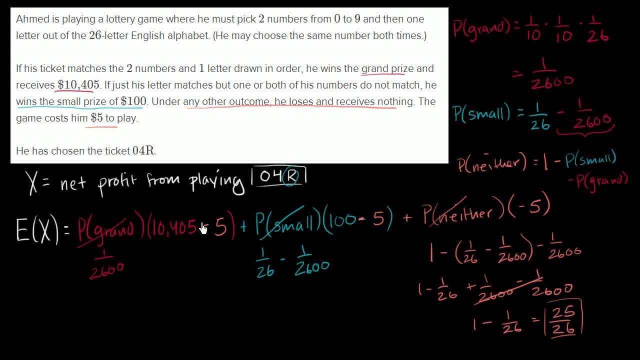 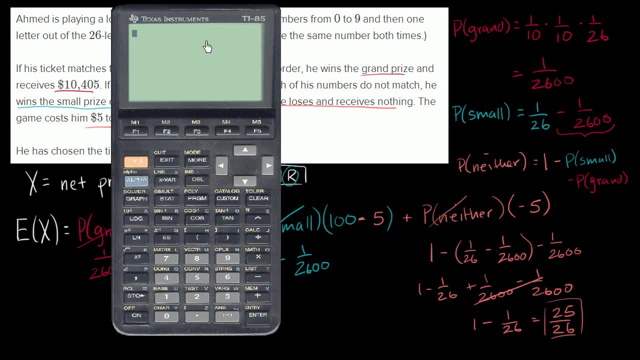 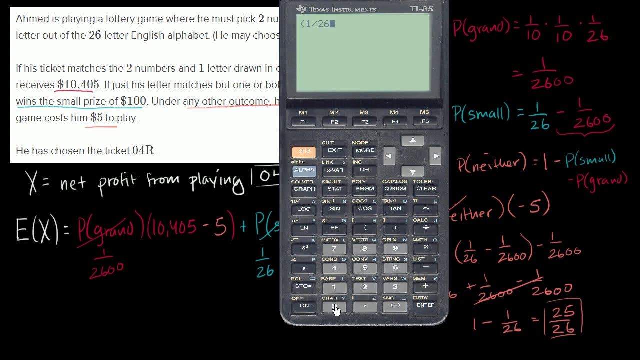 So let's just kick our calculator out And calculate this And we'll round to the nearest. We'll round to the nearest penny here. So let's see, It is going to be 1, 2600.. So 1 divided by 2600. 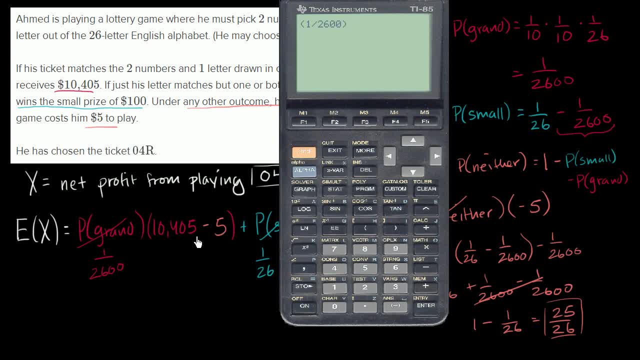 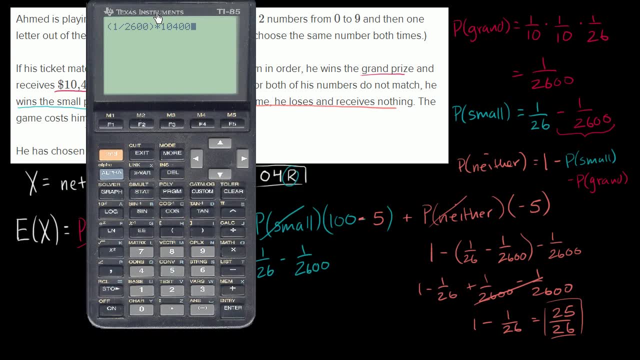 Times Let's see: 10,405 minus 5 is going to be 10,400.. Times 10,400.. That's your net profit When you win the grand prize, And then you're going to have Plus.